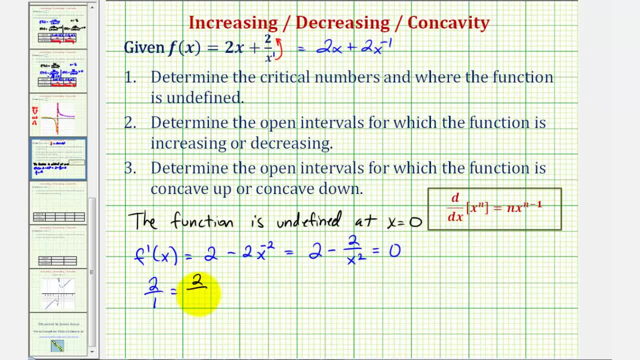 or two over one, equals two divided by x squared. and now we can cross multiply to solve for x, meaning two times x squared must equal one times two. Well, two times x squared equals two. we divide both sides by two, we have x squared equals one. 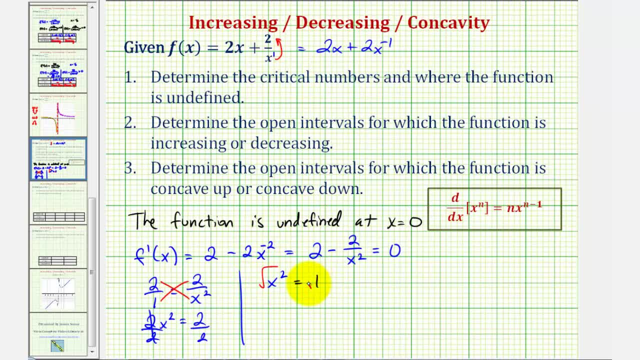 so now we'll take the square to both sides of the equation. we'll have two solutions here. x is equal to positive one or negative one, or plus or minus one, which means we have two critical numbers: x equals negative one and x equals positive one. 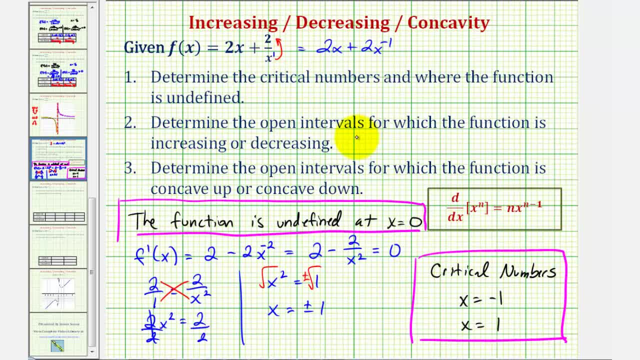 And now for step two. we'll determine the open intervals for which the function is increasing or decreasing. To do this, we'll divide the domain of our function, which we know excludes zero, using the critical numbers and then test the sign of the first derivative. 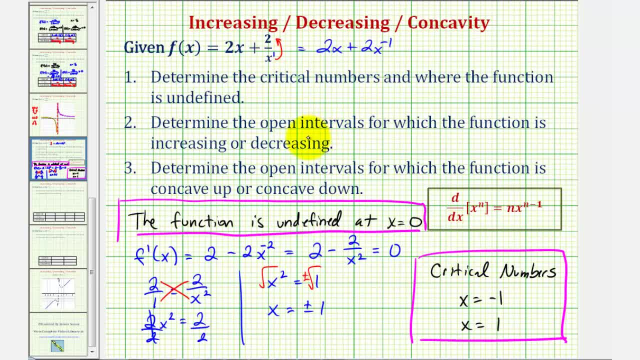 in each interval. If the first derivative is positive, the function is increasing over the interval. If the first derivative is positive, the first derivative is negative, the function is decreasing over the interval. Let's go ahead and set this up on the next slide. 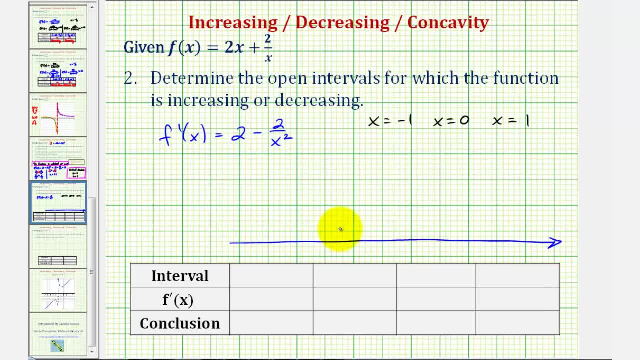 So, if we consider all real numbers, we divide this into subintervals, using where the function is undefined and the critical numbers. we would divide it here at negative one, here at zero and here at positive one. So we'll have four intervals to check. 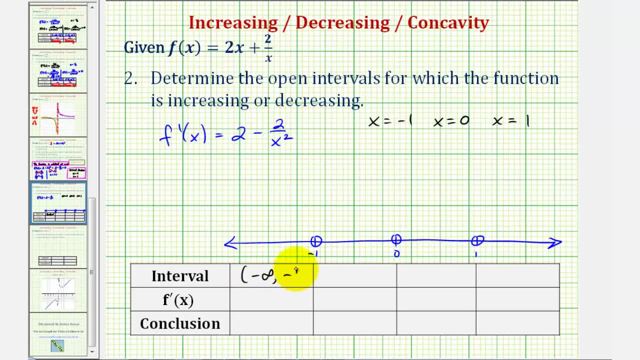 The first interval will be the open interval from negative infinity to negative one, then the open interval from negative one to zero, then from zero to one, and then from one to infinity. So now we'll pick a test value in each interval to determine the sign of the first derivative. 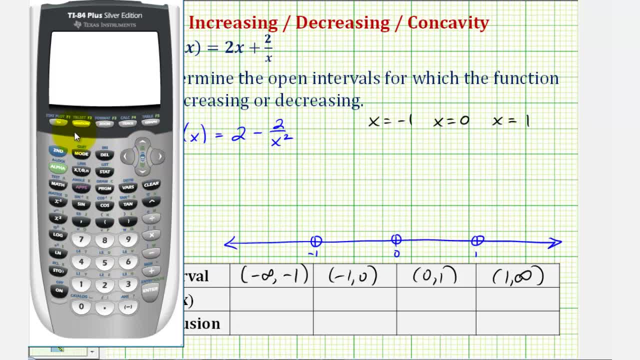 And let's use the graphing calculator to do this. First we'll enter the derivative function into y one, so we'll press y equals and we have two minus two divided by x squared. And now we'll go back to the home screen. 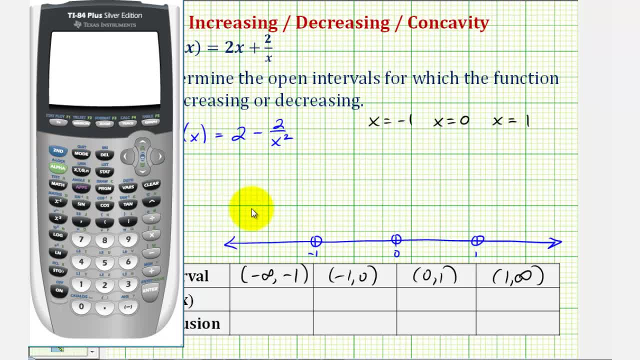 by pressing second mode for quick, and then we'll go back to the home screen by pressing second mode for quick, and then we'll go back to the home screen by pressing second mode for quick and after we determine the sign of the function value. 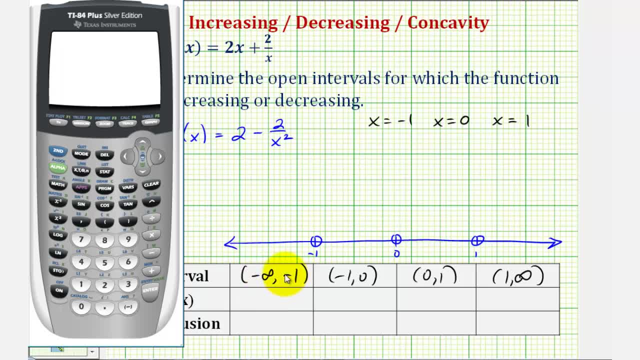 in this first interval. let's determine the derivative function value at x equals negative two. To do this, we'll enter y, one of negative two, So we'll press vars right arrow, enter. enter then in parentheses: negative two. 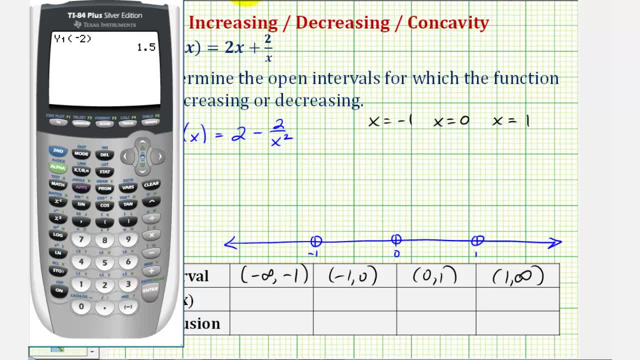 We only care about the sign and notice how it's positive. And now for the second interval. let's test. let's say negative point five or negative one half. So again, we'll press vars right arrow- enter- enter. 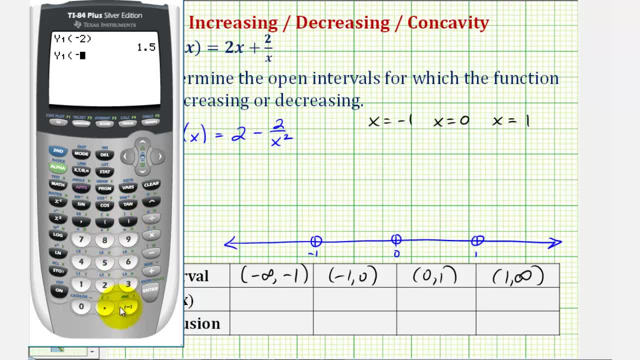 and in parentheses, negative one half or negative point five, Close parenthesis enter. Notice how the sign is negative. So the first derivative is negative over this entire interval. Next we'll test. let's say x equals one half, So again vars. right arrow- enter- enter. 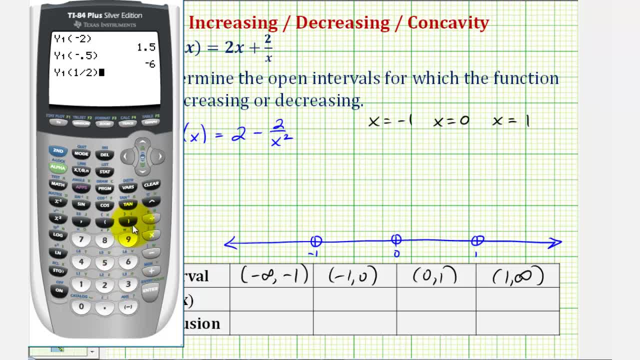 in parentheses one half or point five. Close parenthesis enter. Notice how it's negative again. And now for the last interval we'll test. let's say x equals positive two. So we'll press vars right arrow, enter- enter. and in parentheses two. 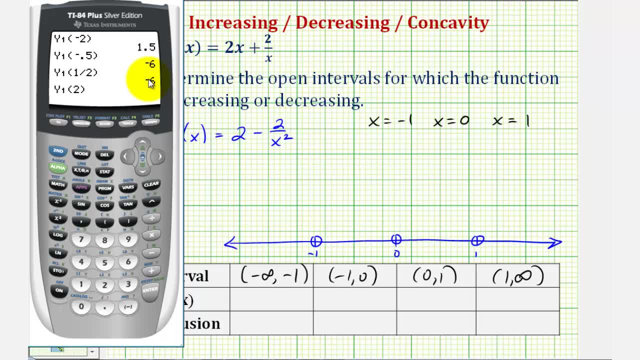 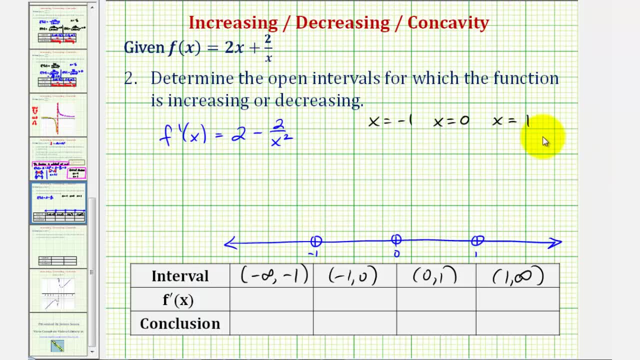 Notice: so far we have positive, negative, negative, and for this fourth interval we have another positive. Let's go ahead and record these results. So it was positive, negative, negative and positive, which means the function is increasing over this interval. 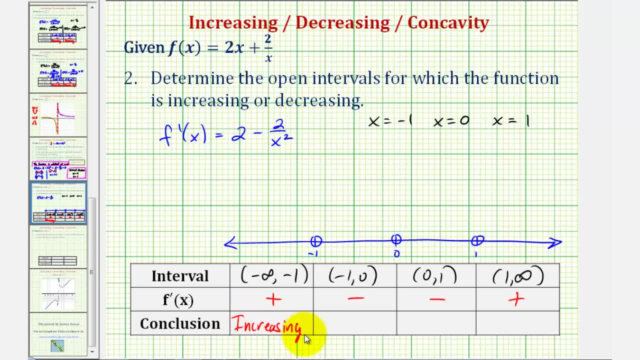 or the open interval from negative infinity to negative one. The function is decreasing over the open interval from negative one to zero. It's also decreasing over the open interval from zero to one And then, following our last interval, the open interval from one to infinity. 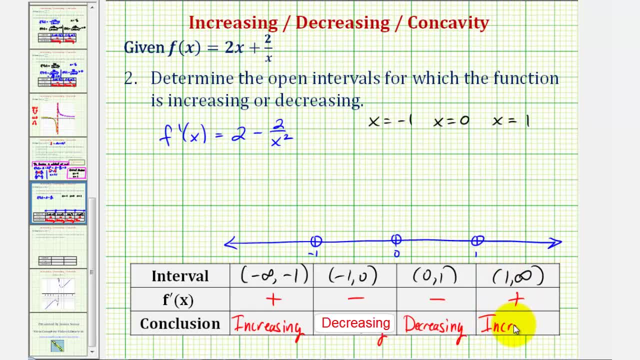 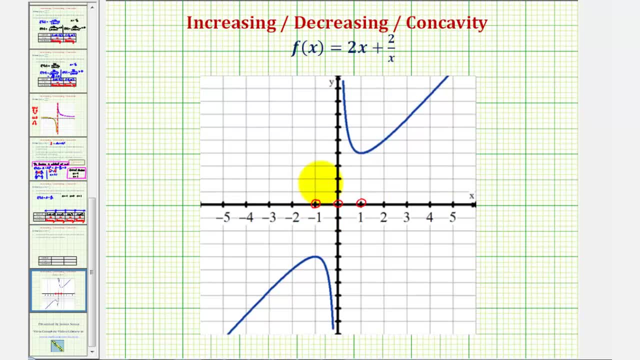 because the first derivative is positive, the function is increasing again. So we can verify these results by looking at the graph of the given function. Notice how, from negative infinity to negative one, the function is increasing as x increases, y increases, Or we can think of them going uphill from left to right. 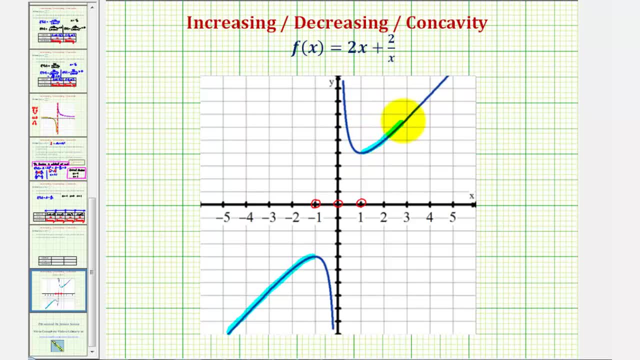 It's also increasing on the open interval, from one to infinity here. But notice, between negative one and zero the function is going downhill or decreasing as x increases, y decreases. and the same thing from zero to one here: as x increases, the y values decrease. 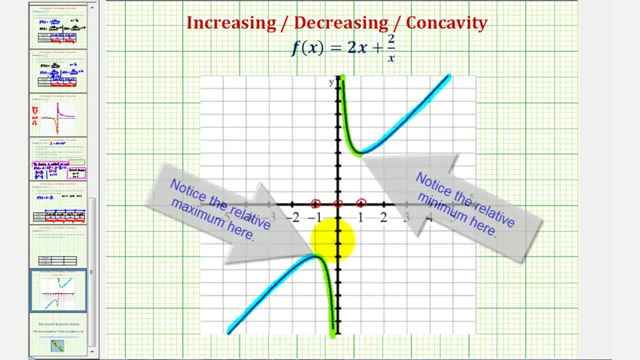 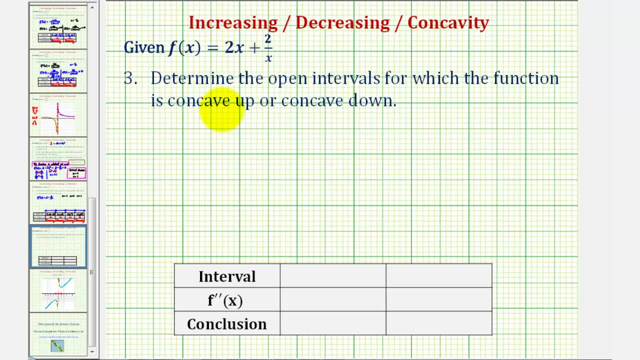 or we're going downhill. So the graph does verify our work. Now let's talk about the concavity of the function. Again, step three: we wanted to determine the open intervals for which the function is concave, up or down. To begin, we'll determine where the second derivative 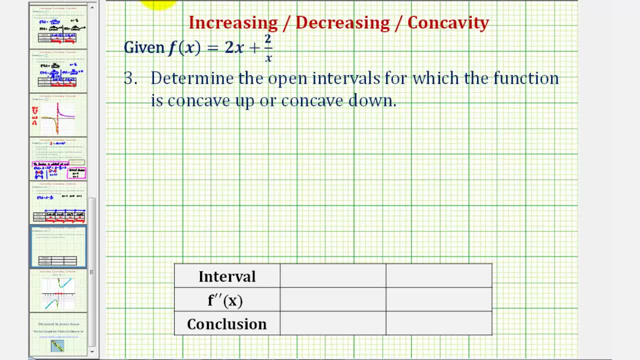 is either equal to zero or undefined. Keep in mind the function was also undefined at: x equals zero And our first derivative function was f. prime of x equals two minus two divided by x squared. which to find the second derivative, we'll write as two minus two times x. to the power. 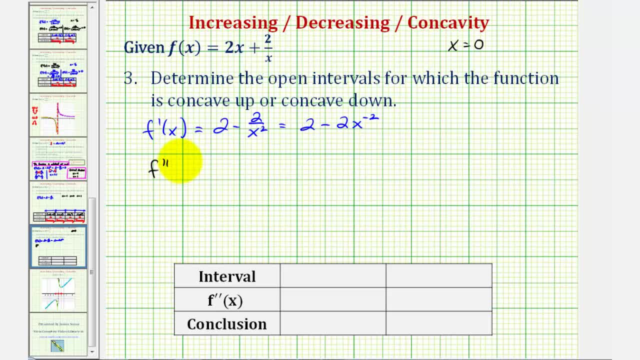 of negative two. So the second derivative function would be the derivative of the first derivative. The derivative of two would be zero For the derivative of the second term. we multiply by negative two, That'd be positive four. Subtract one from the exponent. 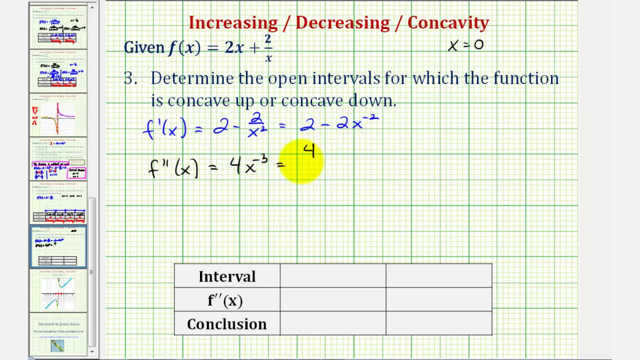 That would be x to the power of negative three Or four. Four divided by x, cubed, We'll notice how this would never equal zero, because a numerator is a constant And it's only undefined when x equals zero, which is also where the function is undefined. 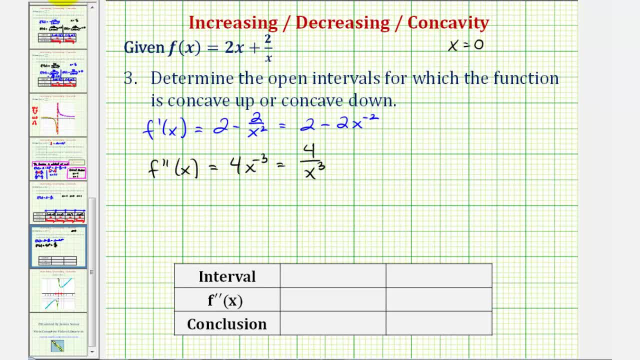 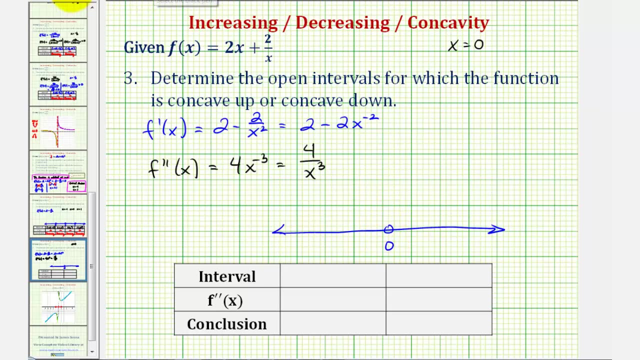 So now we'll divide the number line only using the value x equals zero. So again, if this is a number line, or all real numbers, we'll divide it using x equals zero here, And therefore the interval on the left would be the open interval from negative infinity to zero. 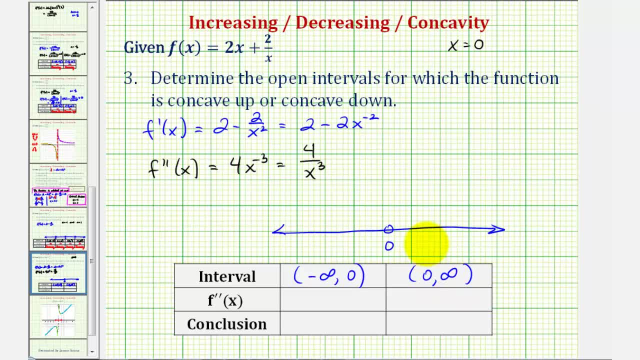 And on the right we have the open interval from zero to infinity. And now we'll check this out on the second derivative, which will tell us whether the function is concave up or concave down. We won't need the calculator for this. 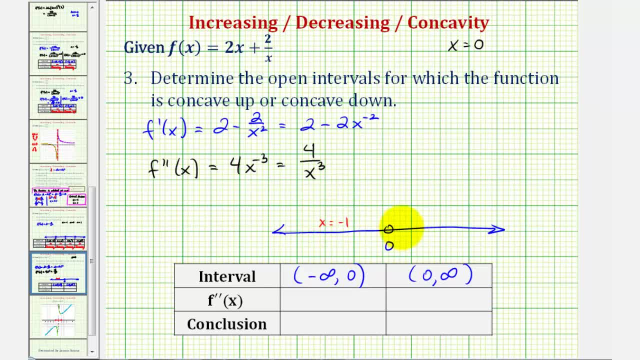 On the left, let's test x equals, let's say, negative one. And on the right, let's test x equals positive one. Well, when x is negative one for the second derivative we would have four divided by negative one, cubed. 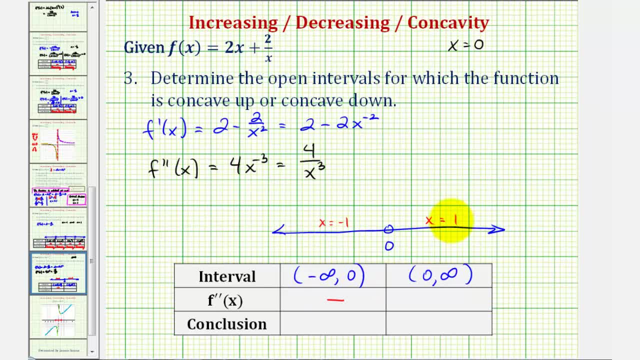 which would be negative four or negative. And when x is positive one, we'd have four divided by one cubed, or positive four, which is positive. So because the second derivative is negative, over this interval, the function is concave down. 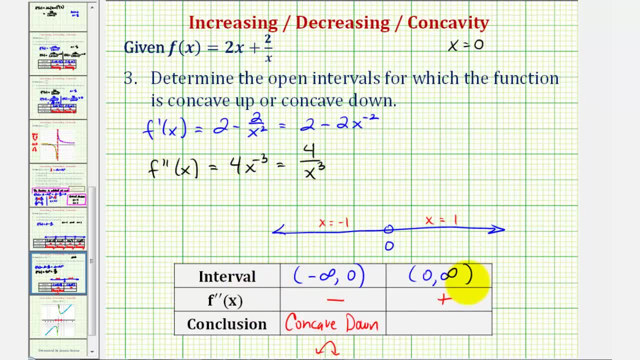 or it would look like this: And the second derivative is positive in this interval, so the function is concave up. or it would look like this: Let's go back to the graph and look, So we can get the left side of the graph.